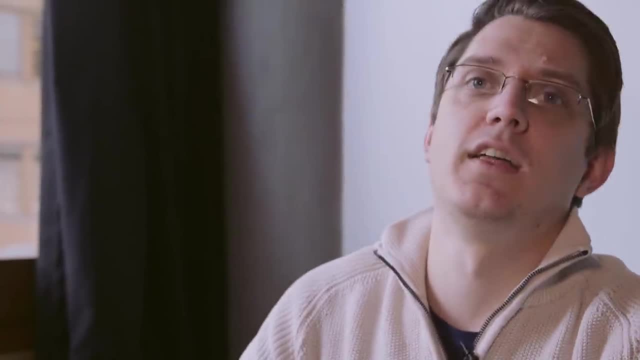 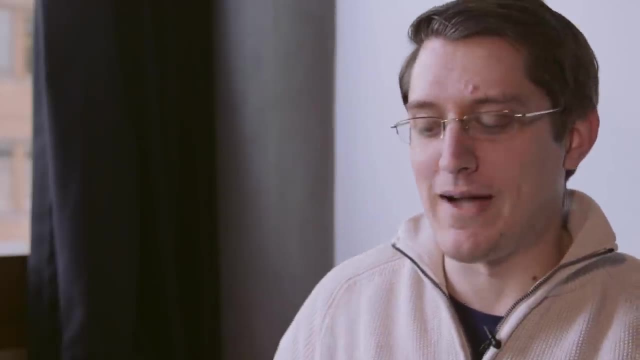 The way that a discrete cosine transform works is: we take some data, in this case our image data, and we try and represent it as the sum of lots of these waves, which doesn't make a lot of sense until you start drawing them out. 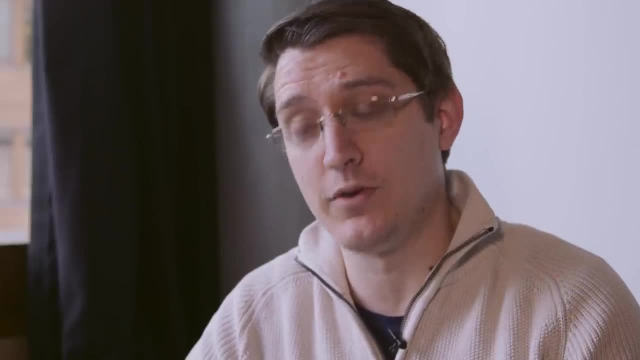 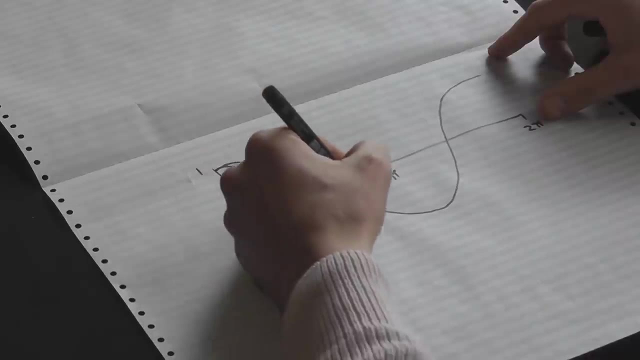 So let's imagine that we've got this cosine wave here, which is our standard frequency cosine, and then we've got another cosine wave which is at a much higher frequency. So that will be: come down a bit faster, go up a bit faster. come down a bit faster and go up a bit faster, like this: 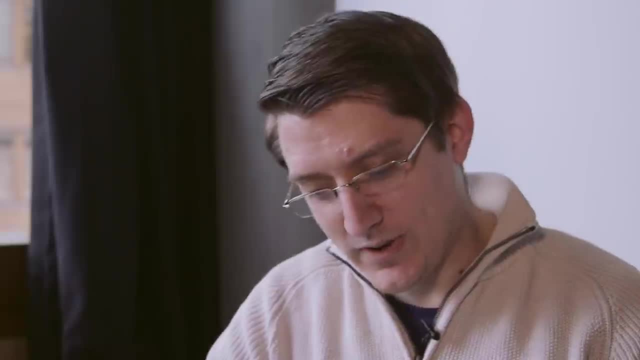 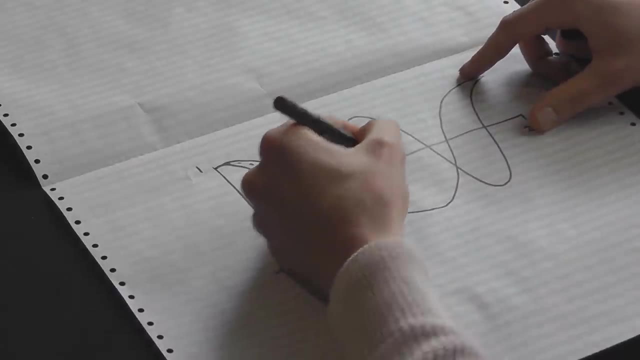 So now we have two waves. If we add them together, what we get is a sort of another wave which is a combination of the two. So if we draw it in here in this dashed line we can see halfway between these two waves is like this: 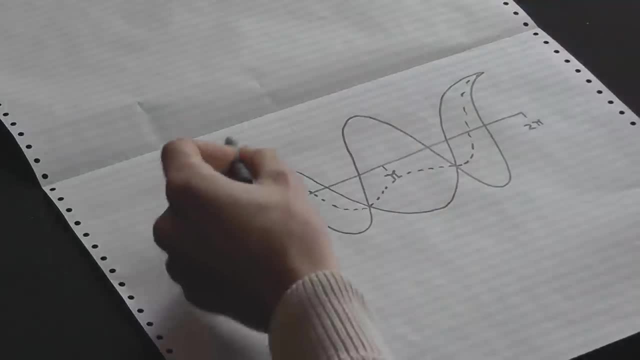 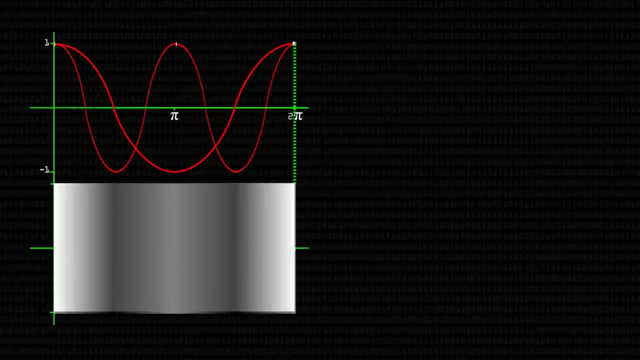 and then kind of like this, And you can see that we've created another, more complex shape, We've created another shaped wave by adding these two together. Now, as we increase the number of cosines, we can increase the number of possible shapes of waves that we can produce. 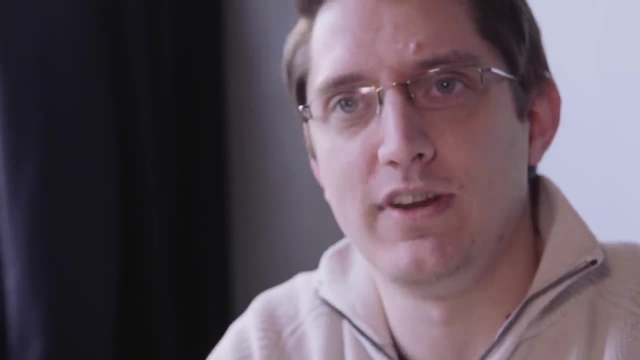 In practice, if we added these two waves together, we'd have a wave that was much taller than the input, So here it would be two not one. So what in fact we do is we weight both of these, and so we take an average. 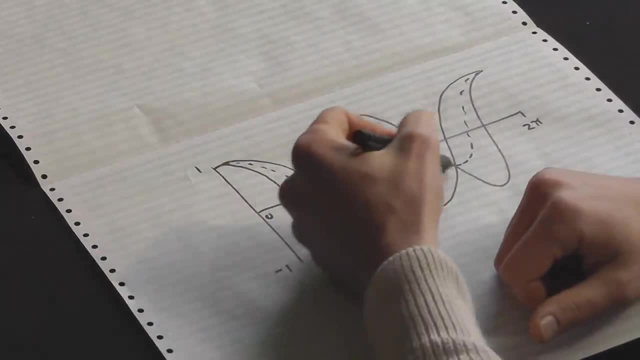 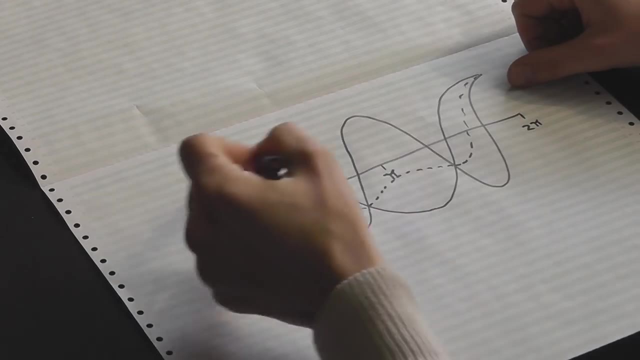 So both of these are weighted, in this case as a half, and so this is essentially the average of both of them. We could also change the weighting of these So we could have: it was mostly this high frequency wave, This low frequency one, but only a little bit of this low frequency one. 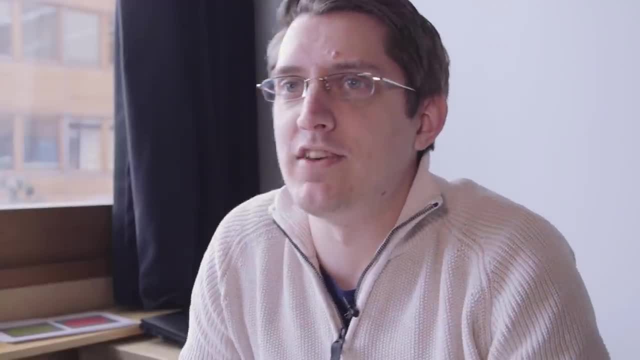 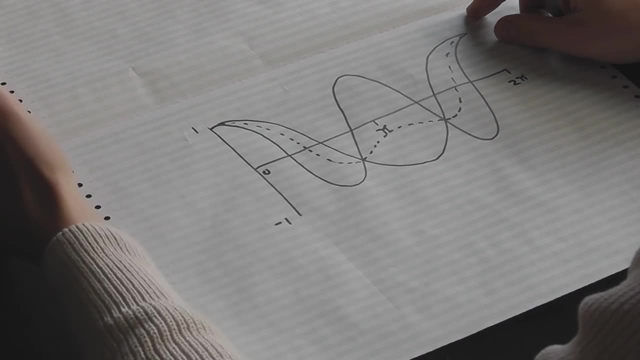 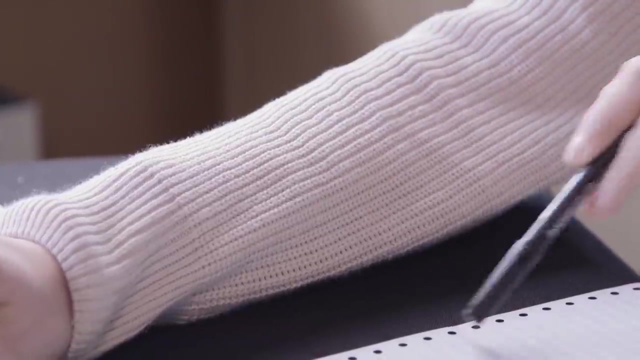 And we'd have a different shaped wave coming out at the end. So each wave represents a small constituent of the output And the higher the frequency of the wave, the higher the frequency part of the signal we're dealing with. So if we look at my jumper here there's a low frequency change from this black table to a brightness right over my jumper to dark table again. 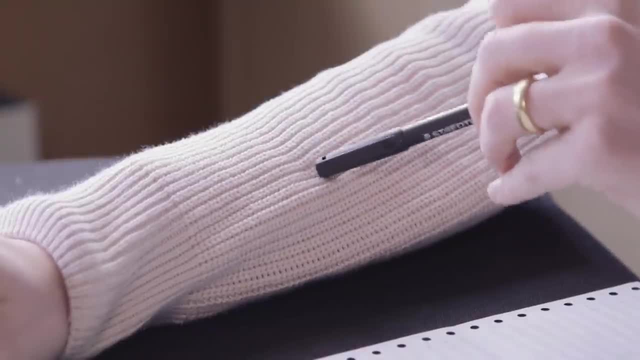 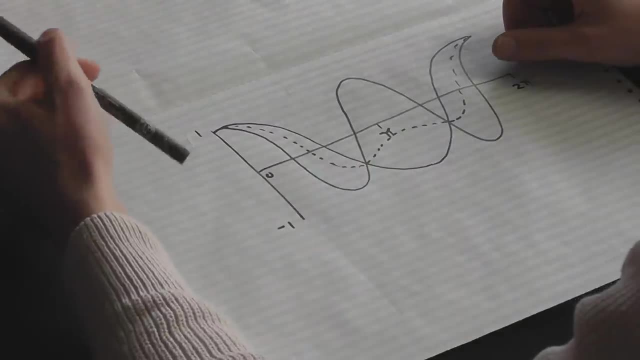 And there's much higher frequency changes on my jumper where we go up and down within sort of the woolen knit, And it's the same kind of principle. So what we're doing in JPEG- that we can get rid of some of the higher frequency signals and the general gist of the image will still be there. 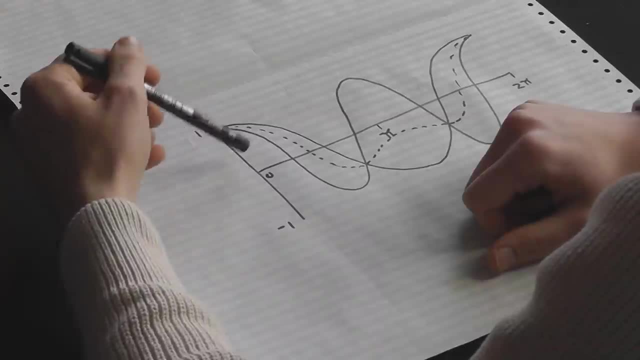 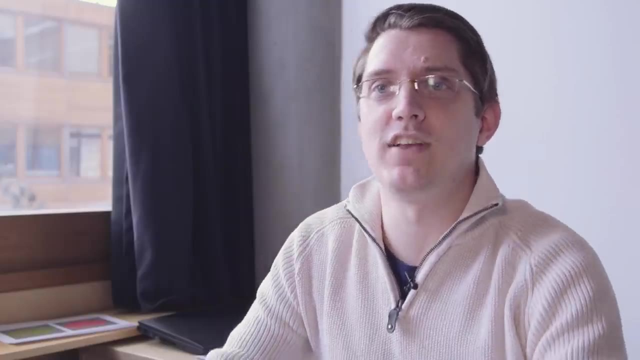 So this is just a one-dimensional, discrete cosine transform with only two components. The way that the mathematics works is: if we have a signal that's eight long, then we find that we can represent it using eight cosine waves of different frequencies, And the same is true of an image. 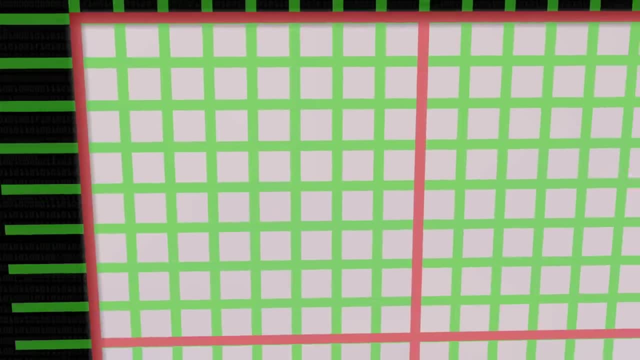 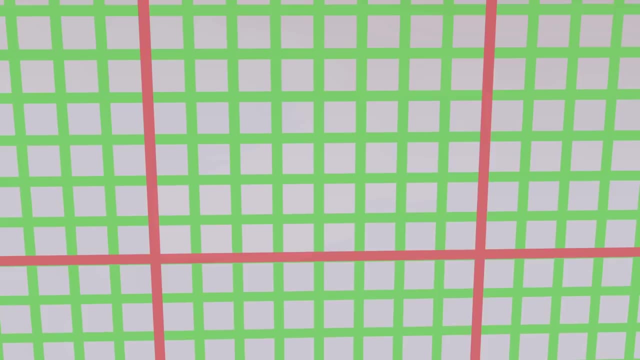 What we do in JPEG is we split each image into eight by eight pixel groups, And each of those pixel groups is separately encoded with its own discrete cosine transform. Each of those eight by eight pixel groups can be exactly replicated by 64,. so eight by eight cosine waves. 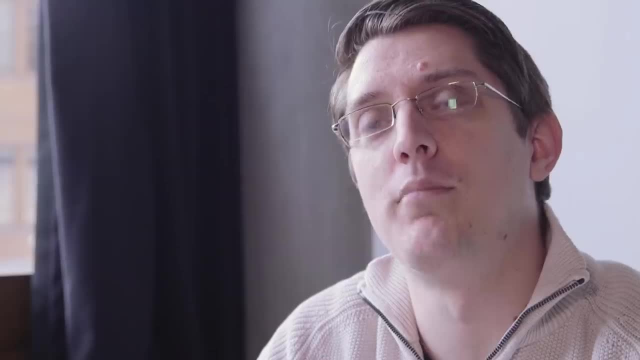 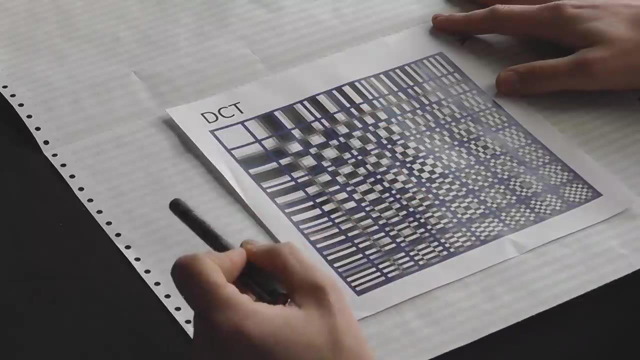 This actually shows the 64 base cosine waves that produce any image we might like to do in eight by eight pixels. This particular component here is essentially flat, So if you had only this component and that was all that contributed to your final output, your image would look like that. 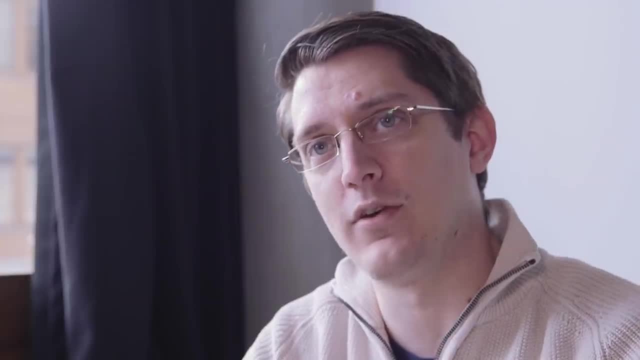 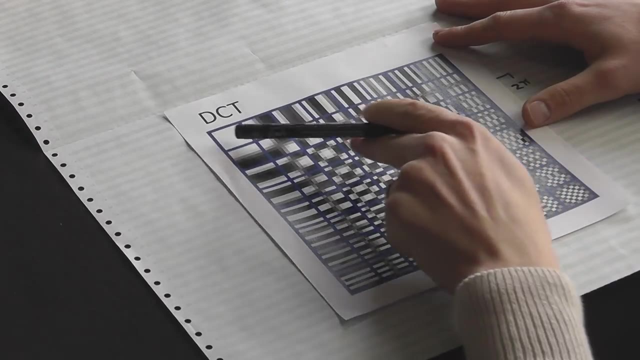 If you had only this one, your image would go white and then it would dip down and go black, And you can see that the frequency is increasing as we go along here. This is in the x direction and then in the y direction. the frequency is increasing down here. 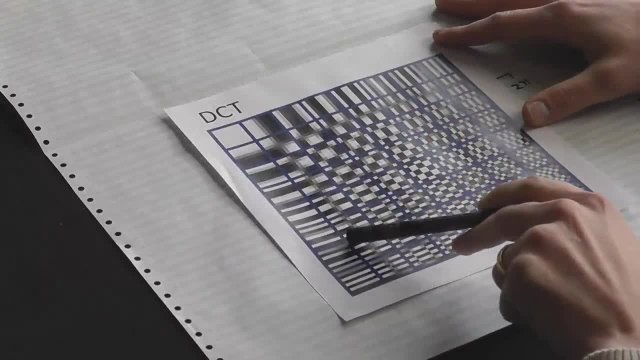 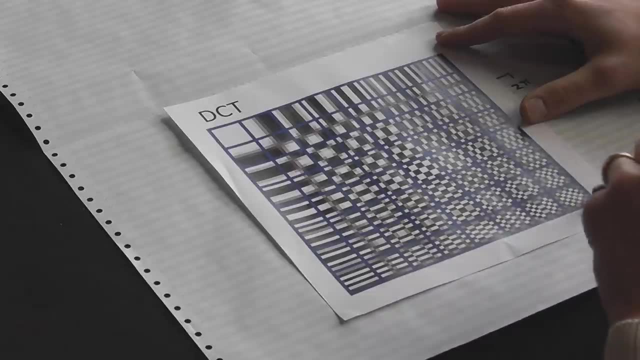 So this is a cosine wave and this is a higher frequency cosine wave down here. As we increase the frequency in both directions, we get a kind of checkerboard pattern And this is a high frequency information that we're encoding in these regions. 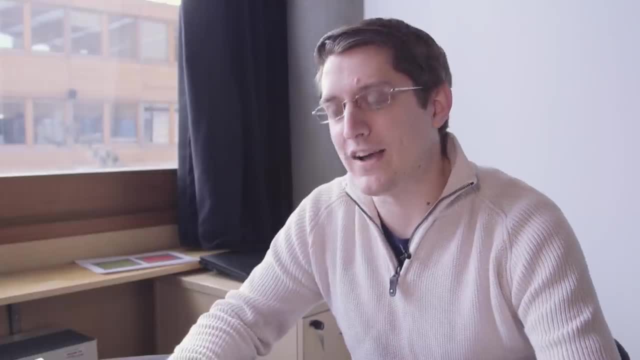 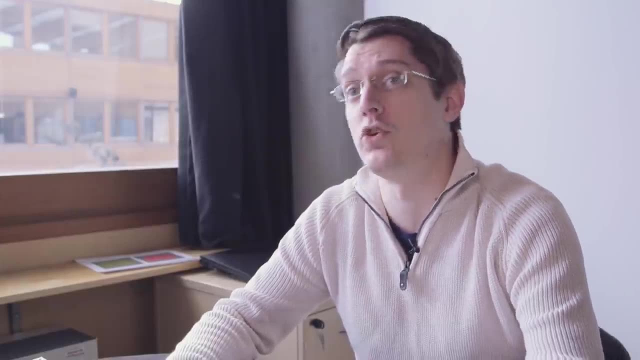 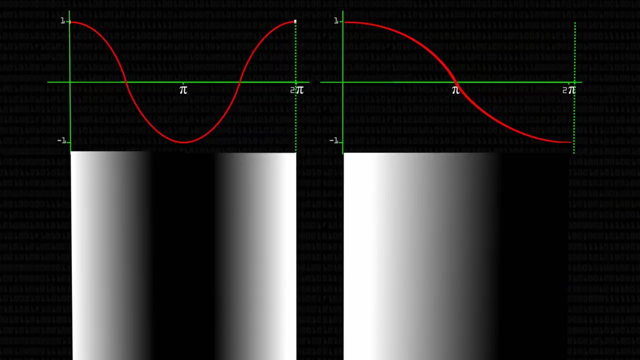 So these are the 64 cosine functions that can be compiled. These are the functions that can be combined to make any eight by eight image. This is only in one channel. so let's say just luminance or just CR. For example, if we had half of this wave and half of this wave, then what you would get is a square of image that was generally brighter on the left with a little bit of bright on the right-hand side, because you've summed the two together. 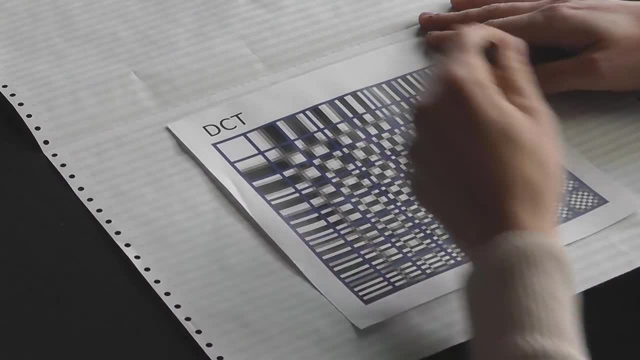 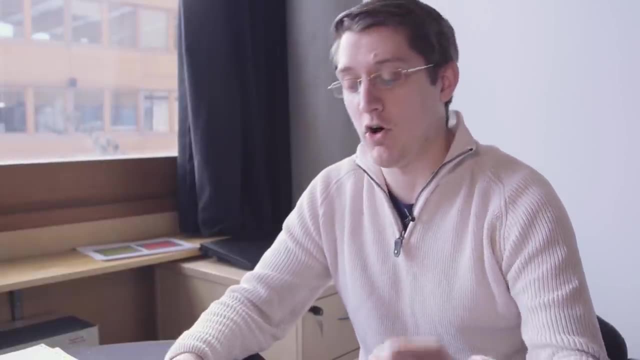 To create any kind of eight by eight image. what we need to do is have a combination of all of these. at the same time, Each of these is weighted based on something called a coefficient. This is a number representing the contribution of each of these individual blocks to the whole. 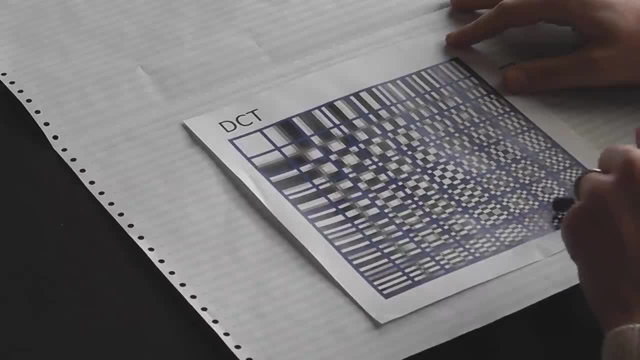 So, for example, if the contribution of this one is zero, then there is no part of this cosine wave in the eight by eight image that we're looking at. If it's a 0.1 and this one's 10, then this has obviously got a hundredfold less impact on your output image than this one. 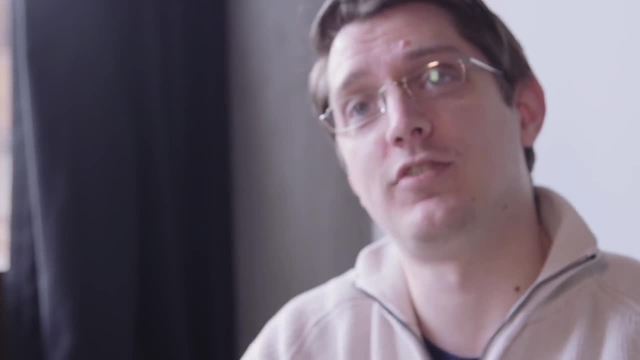 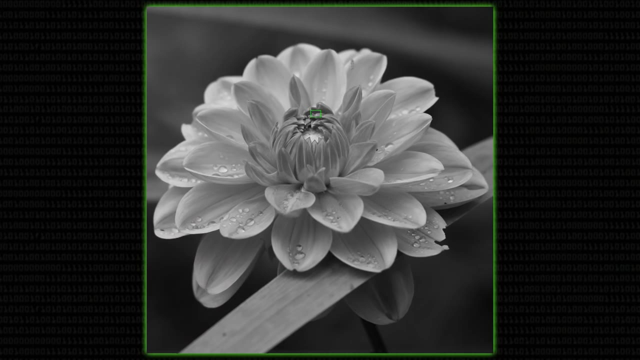 And what we do with a discrete cosine transform is basically calculate the coefficients for these waves. Putting this discrete cosine transform aside for a minute, let's look at an example image. So this is a small crop section of our flower image. This is the y component. 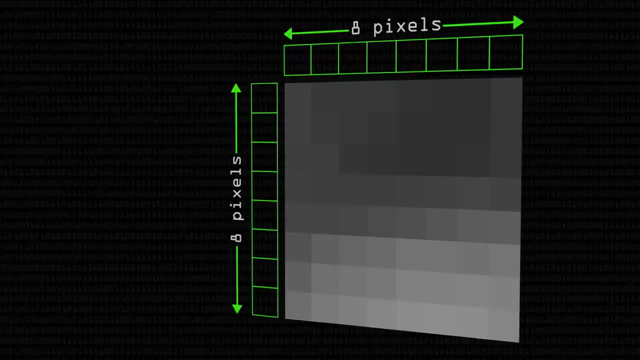 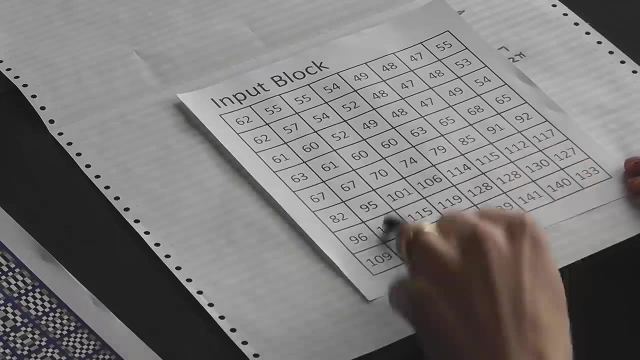 So it's just every value from 0 to 255.. How intense is the pixel? So you can see this is not a hugely interesting piece of image. It's kind of gray with a little bit of brighter region down here. What we want to try and do is calculate the contribution of each of our cosine waves to this image. 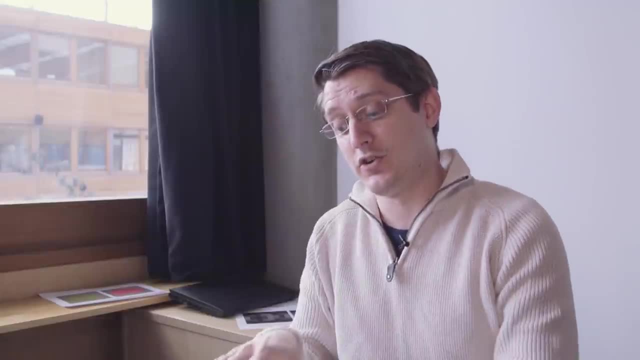 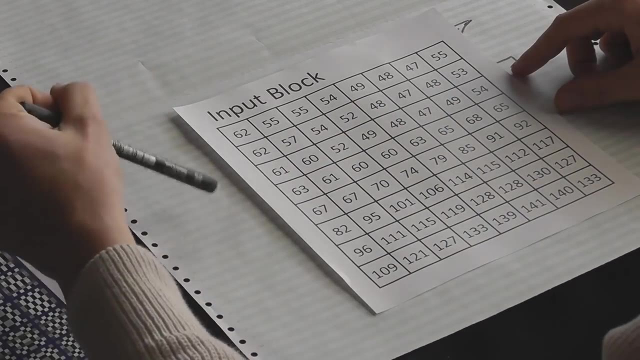 Which bits of cosine do we need to add together to create an image that looks exactly like this? So, to start with, what we need to do is center all of these values, which are currently centered around 128, because they're from 0 to 255.. 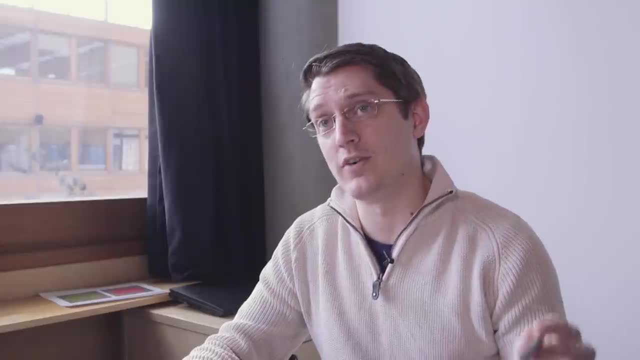 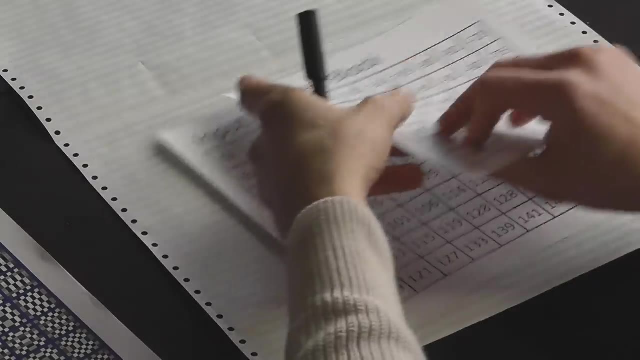 We center all these values around 0 because, remember, a cosine wave goes from 1 to minus 1, not from 1 to 0. So we take away 128 of every value and we get our shifted block like this. So this is the exact same image, but this time now centered around 0.. 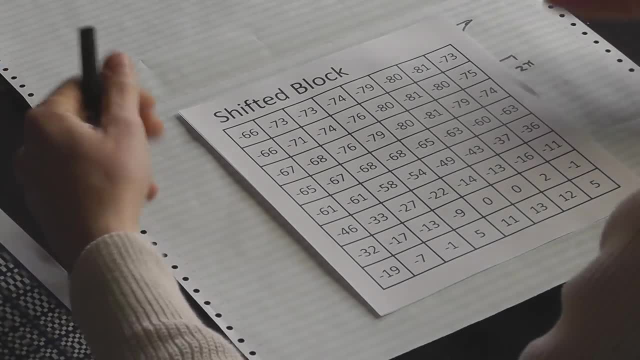 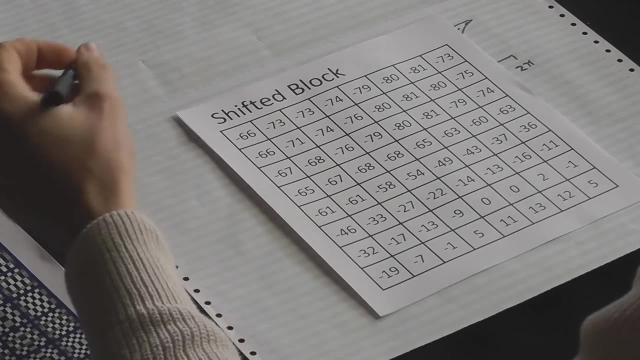 And now we can use this in the discrete cosine transform to calculate our coefficients. We apply the- it's actually discrete cosine transform, number 2, which is the one that's always used in JPEG, And what that does is calculate the contribution of each of our cosine waves. 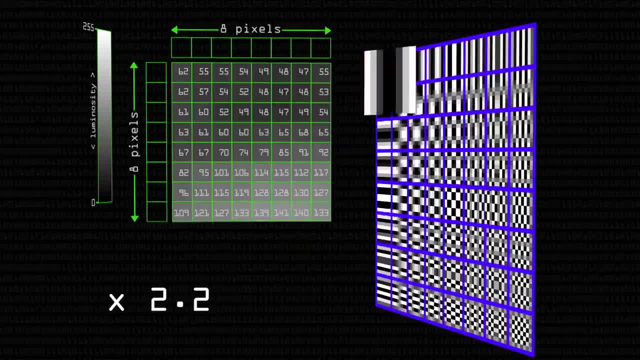 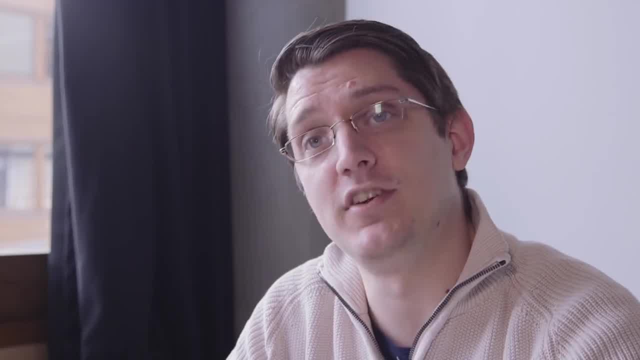 that, when added together, will create this image exactly right. Which of these blocks, when multiplied by their coefficients to tell us how much of each one we use, will add together to create this exact image? So it might be a bit of that, a bit of this, a bit of that, a lot of that. 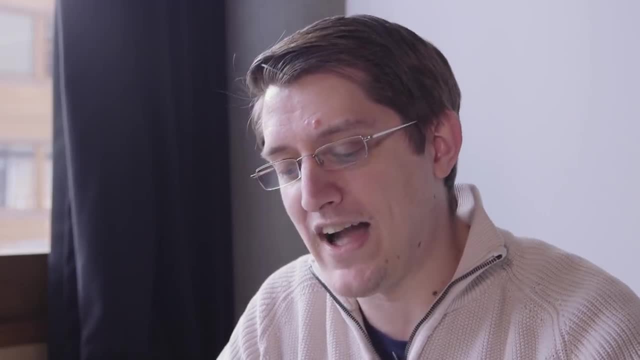 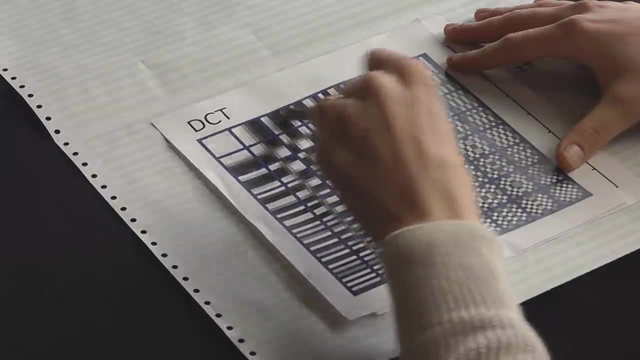 Yeah, and none of this one exactly, And so you'll find that all of these will have some impact on the image, It's almost certain, unless the image is completely flat. One of the nice things about JPEG is these low frequency ones will have a much bigger effect. 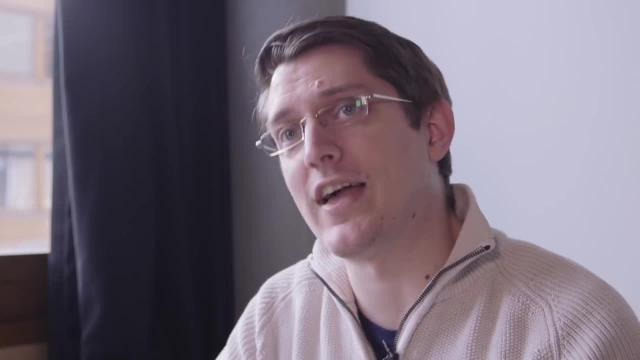 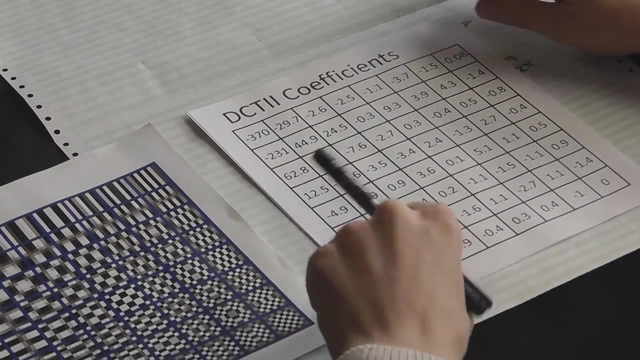 than the high frequency data, And we also see them better. So that's how we compress JPEG. So we calculate our DCT2 coefficients and that gives us some slightly arbitrary values between minus 1024 and plus 1024.. But that's not too much of a big problem. 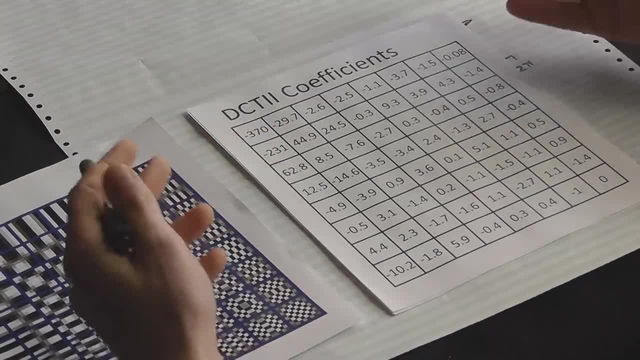 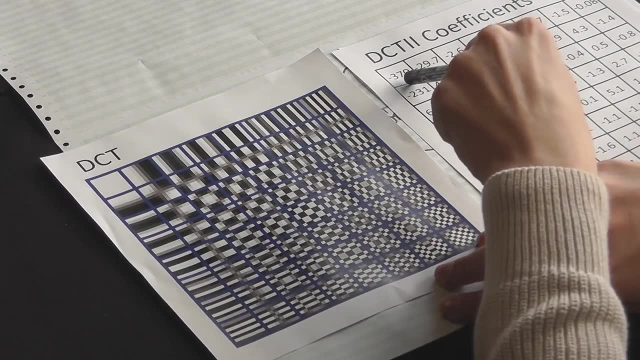 And what we have. each of these represents the weight or the amount of each of our cosine waves. So if we put this next to here, we can say that if we take this cosine and multiply it by minus 317, and add it to this one, multiply it by 29.7,. 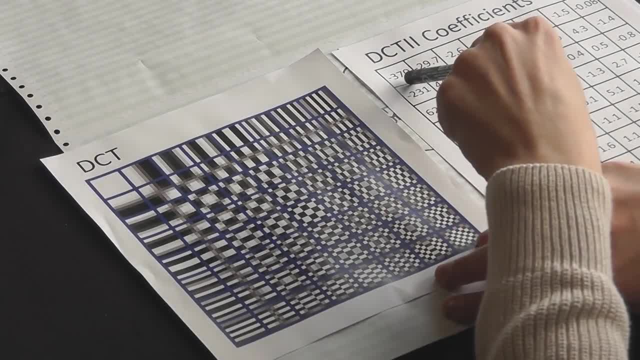 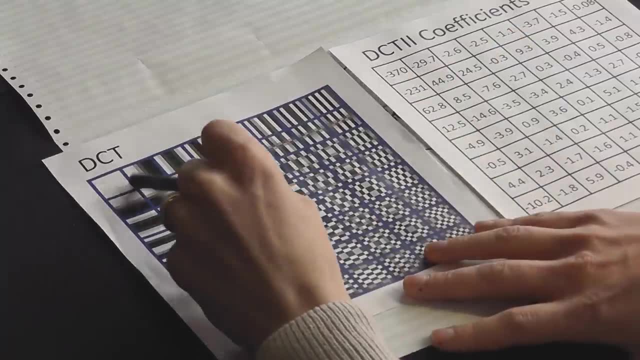 and so on, and we do it for all of them. the added sum will be our original image back again. Usually, this top left coefficient is much bigger than the others Because it's a flat- and it's actually flat and not a cosine wave. 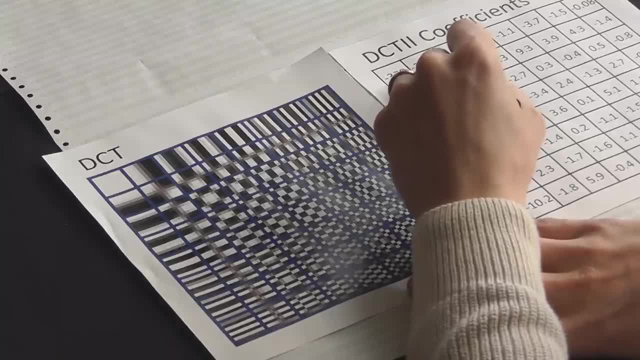 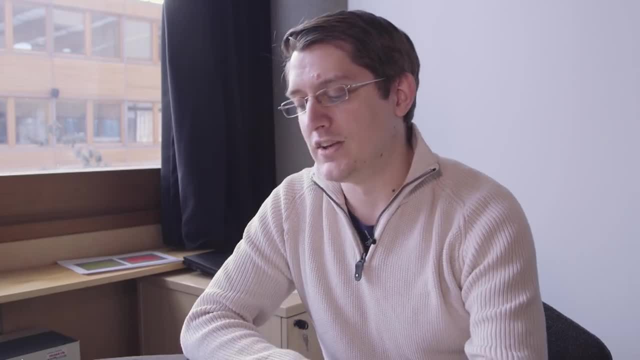 it represents the general intensity of that particular image block. So this is called our direct current coefficient, our DC coefficient. All of the others are alternating current AC coefficients. In practice usually the DC coefficients are stored separately, But we won't dwell on that too much. 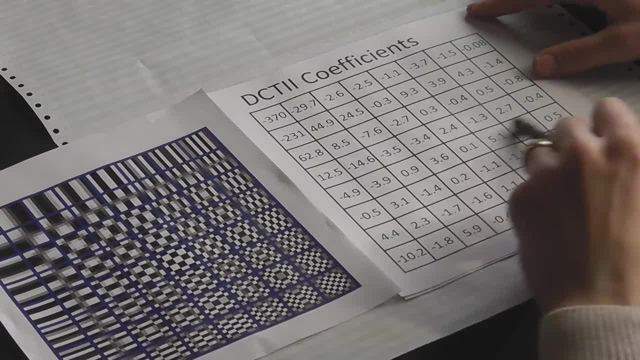 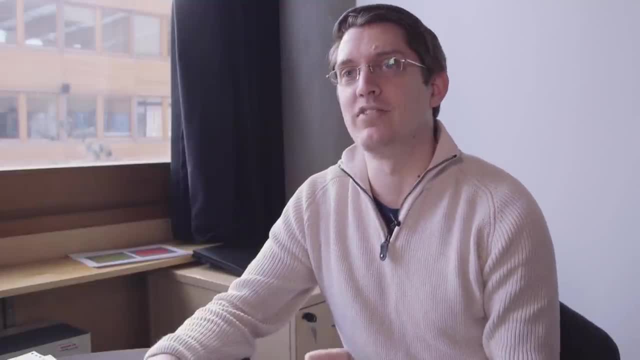 The really important aspect of JPEG that you want to understand is that these coefficients are often very, very small, And these ones are very, very big, And what that tells us is that the high frequency cosine waves don't really contribute very much to the image. 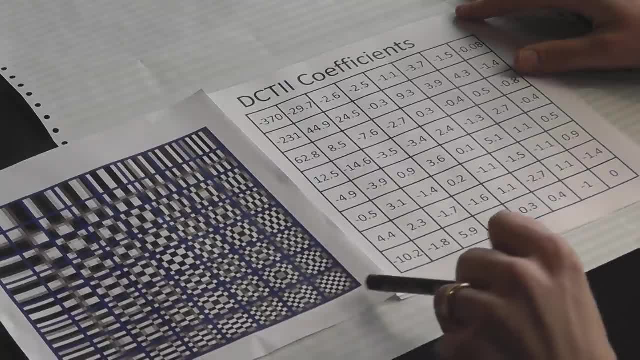 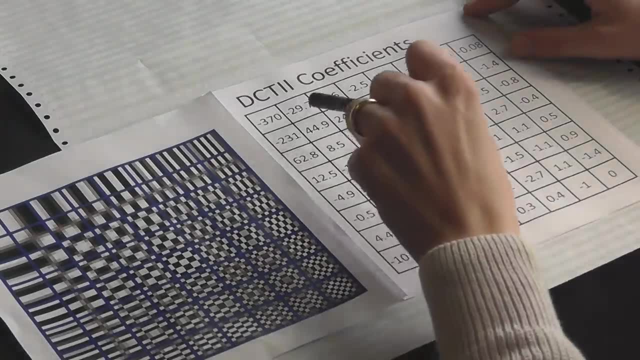 For example, this one is zero, which means that this cosine wave here is having no effect on the image at all. The image is essentially not a checkerboard in any way. These ones, compared to these big coefficients here, are incredibly small as well. 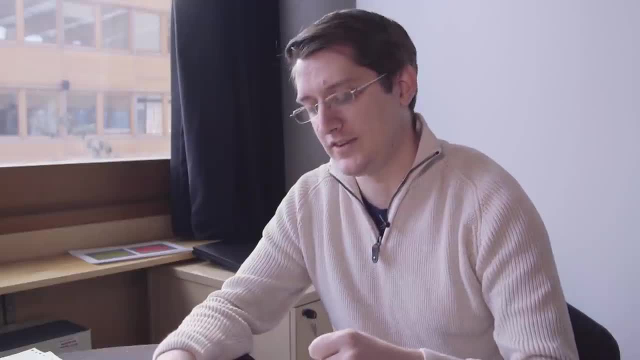 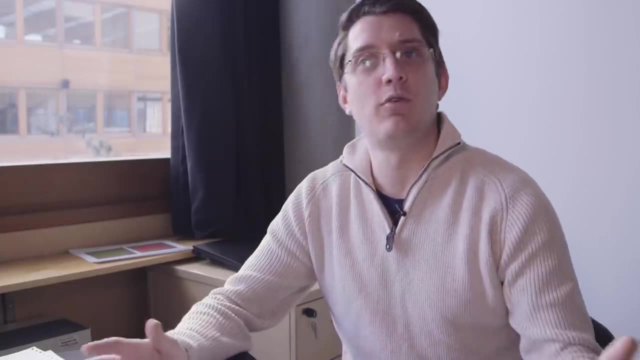 and have very subtle effects on the actual output. pixel data. I mean, these weights are so small, but if you took these away, the image would be almost identical, And yet we could just take them away and save all that space. So that's how we do it. 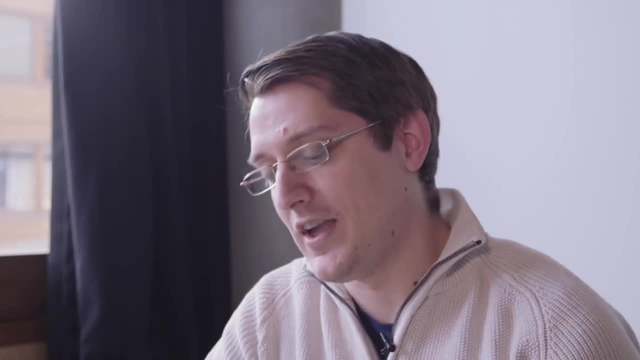 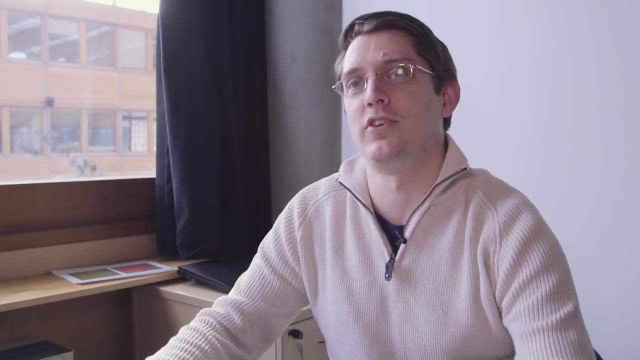 The next step, after calculating our discrete cosine transform coefficients, is to basically try and remove the ones we don't want. We call the process of removing the high frequency data quantization. Hopefully, it'll be easier if I show you a quantization table. 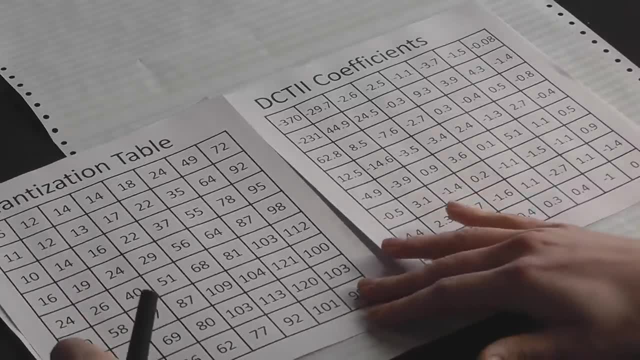 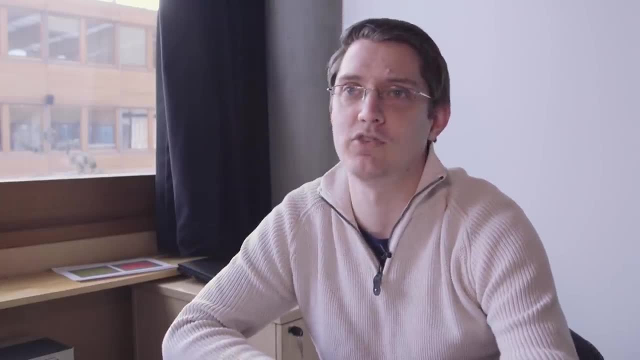 This is the standard JPEG quantization table that represents a quality of 50%. so in the JPEG standard Different compressors, like the one used in Photoshop, will use different quantization tables depending on how they feel and also what level of quality you set it at. 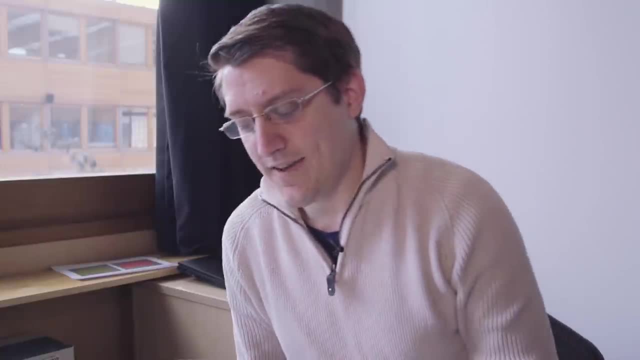 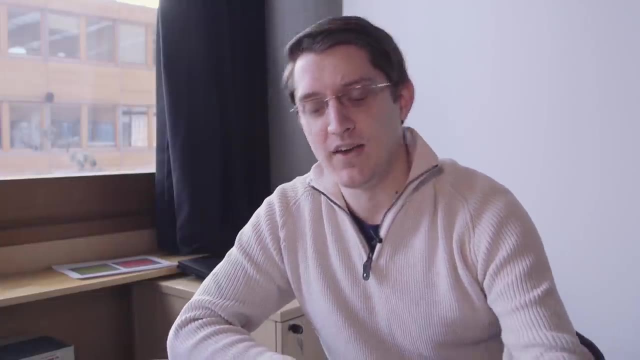 And what we do is we divide every one of our coefficients by the corresponding quantization value and then round to the nearest integer. Okay, And you can see already that these ones are much bigger than these ones. So what essentially happens is these get scaled by a huge amount. 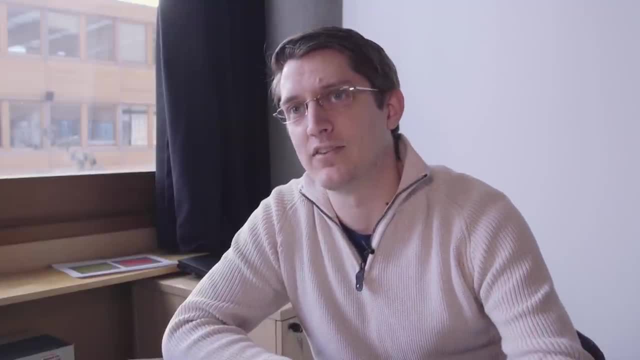 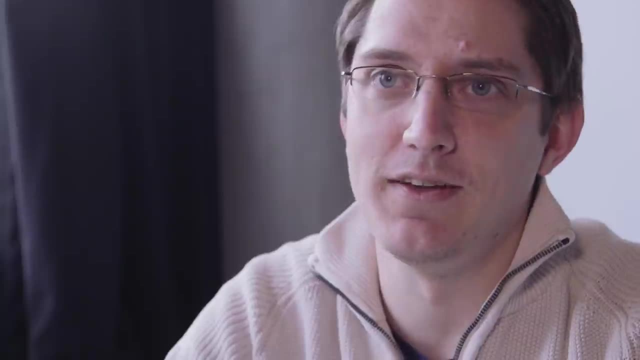 usually to close to zero and then get removed by being set to zero when we round to the nearest integer. So, for example, 370 divided by 1, divided by 16, is roughly 23,, or minus 23. And the actual quantized output is this: 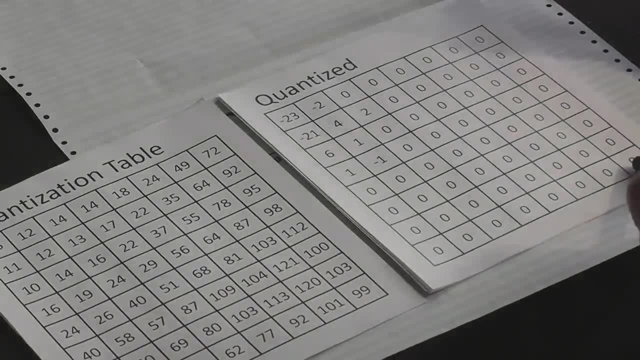 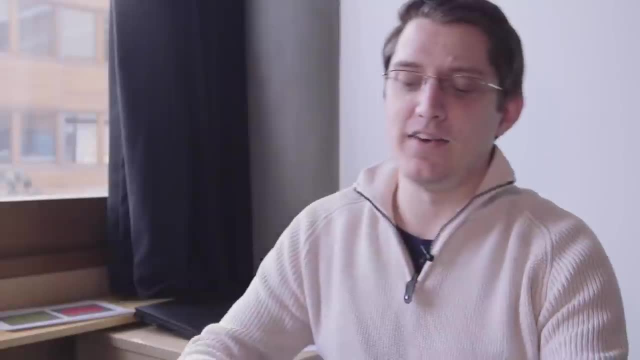 And you can see that almost all of it is now zero. So this coefficient now no longer has an effect, nor does this one or this one. The only ones that have any effect on our image are these nine here And essentially the argument that we're making. 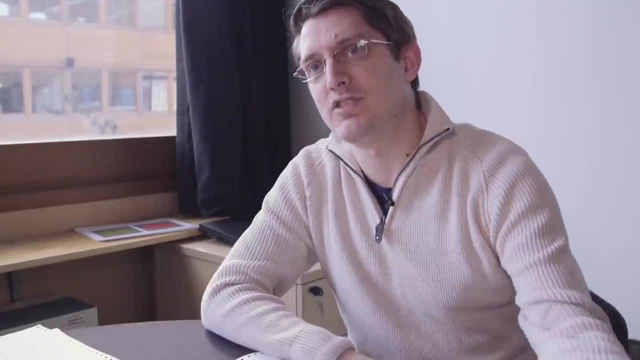 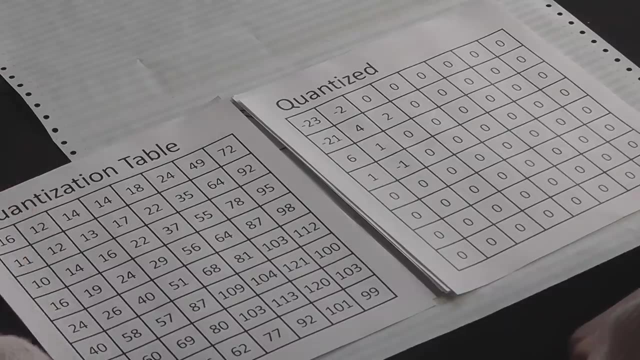 is that with just these nine we can get pretty much the exact same image back. It won't be exactly the same. A couple of pixels will be, maybe an intensity level up or down, but when viewed at a normal image range, you know, let's say a photograph or on a monitor. 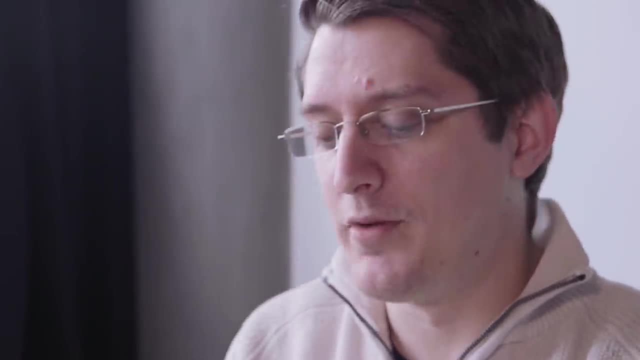 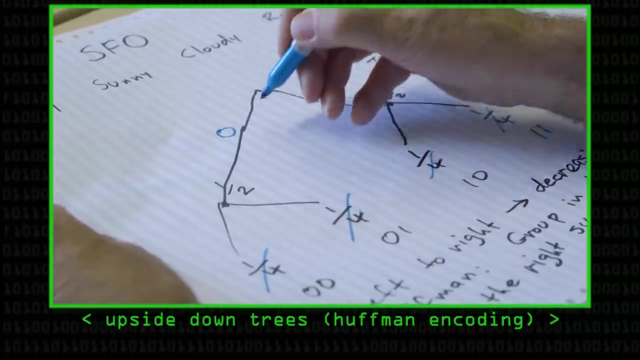 it'll look exactly the same to us. So what we then finally do, when we want to output this information into our file, is we essentially list all these in a long line. We then use a Huffman encoding, which Professor Brelford has covered in a video. 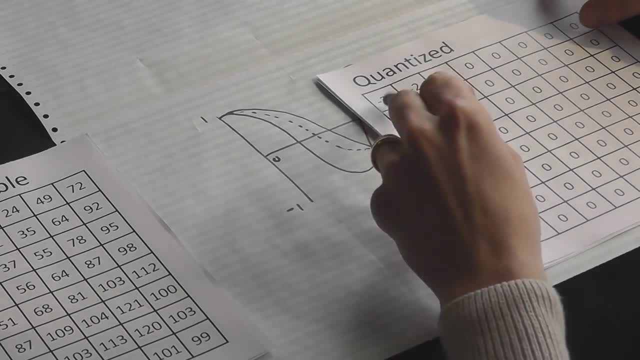 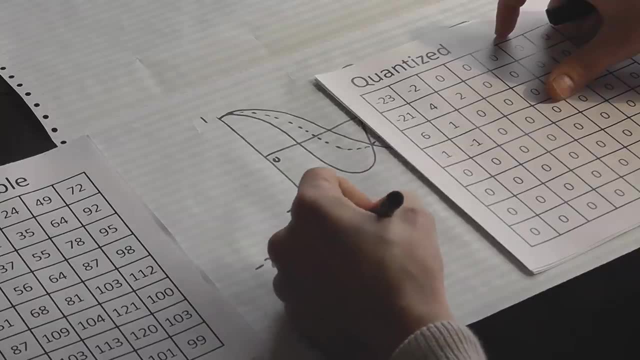 to further compress this data. The way that we serialize this into our file is in a zigzag fashion. So we start with minus 23,. then we go minus 2,, minus 21.. So we're going up and down, and up and down. 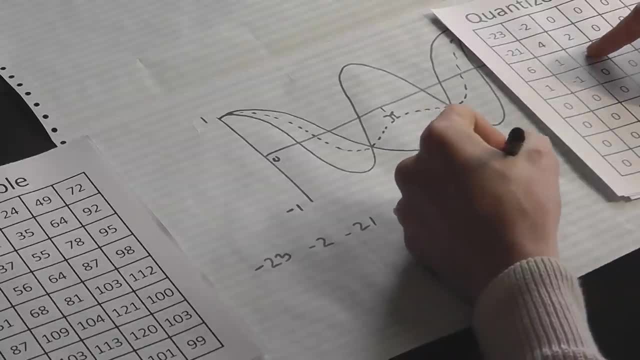 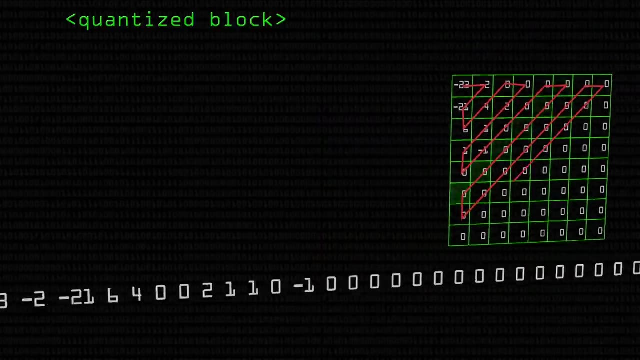 6,, 4,, 0,, 0,, 2,, 1, and so on, And the important thing about this is: by doing this, we're going to get a huge list of noughts all in a row, And that is very easily compressed by Huffman encoding. 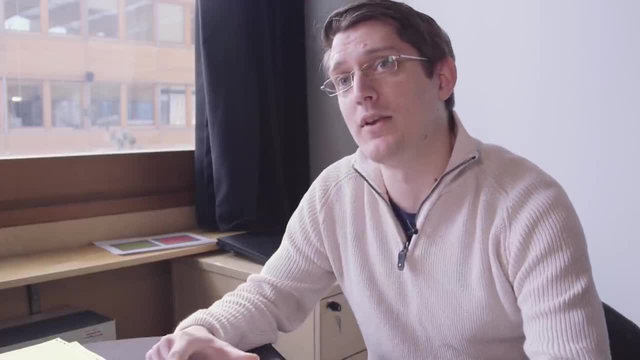 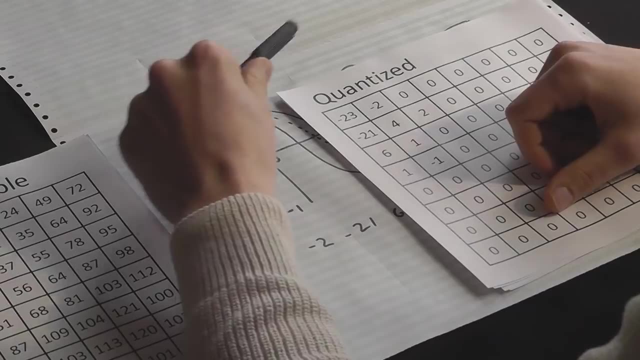 So we take this table and we do this for every 8x8 block in our image. We then serialize them out into a long line and we use Huffman encoding to shrink them right down, and that's what goes into our JPEG And then all other aspects of JPEG. 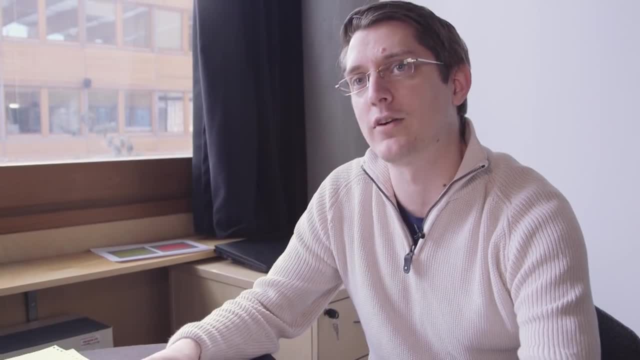 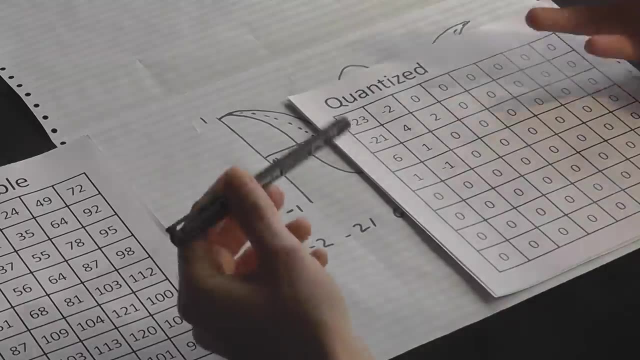 are really sort of minor format considerations. That's the core of how the compression works. To decompress the image. let's imagine that we've sent our JPEG to someone and their decoder is trying to read it. What we have to do is the exact opposite of this approach. 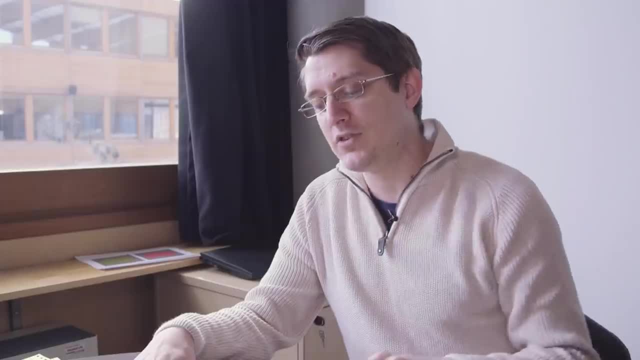 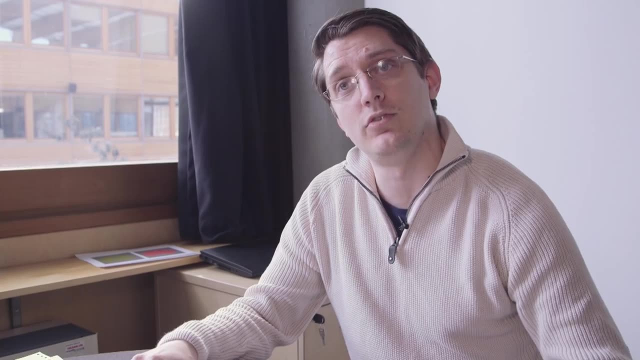 So we begin by multiplying each of these values by our quantization table. So this is the same quantization table. It's stored inside the JPEG, so we know which one they used, Because if you use a different one on the way out, you're going to ruin your image. 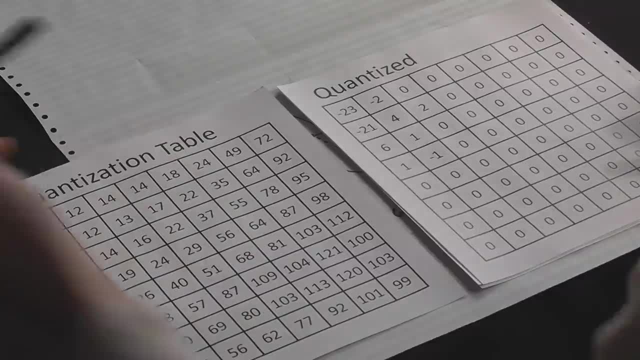 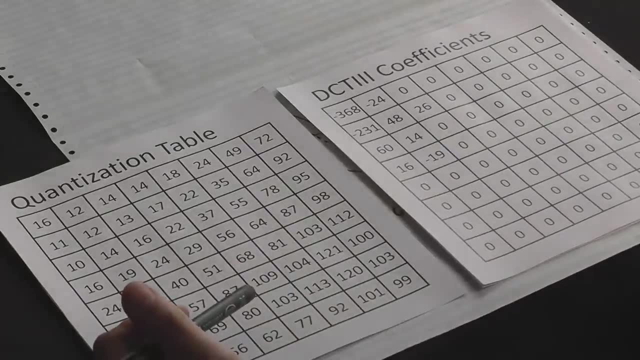 So we multiply each of these values by the specific value in the quantization table and we get the coefficients. And you can see that because most of them are nought, most of them on the other side are also nought. So none of these are going to contribute to our image anymore. 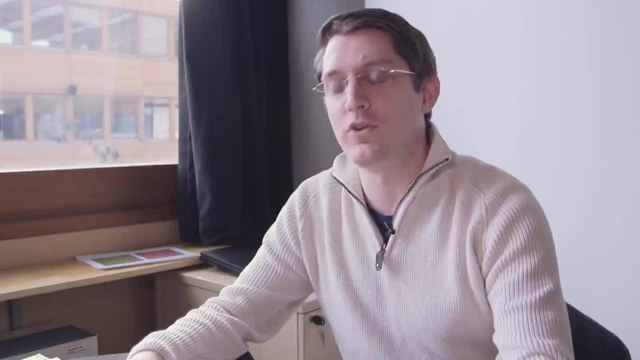 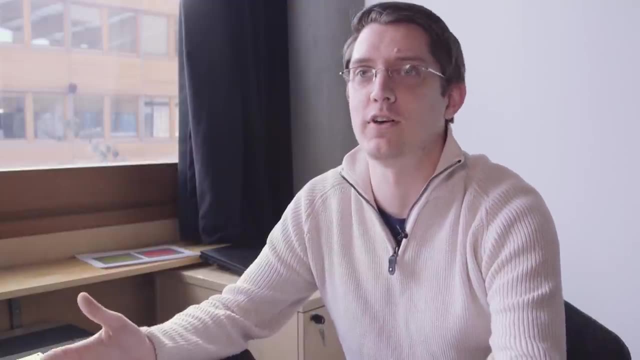 Then, in reverse, we use discrete cosine transform number three, which is usually just called the inverse discrete cosine transform, because it's generally used to inverse what we did for discrete cosine transform two, And that gives us our shifted block back again, which, of course, we then add 128 to every value. 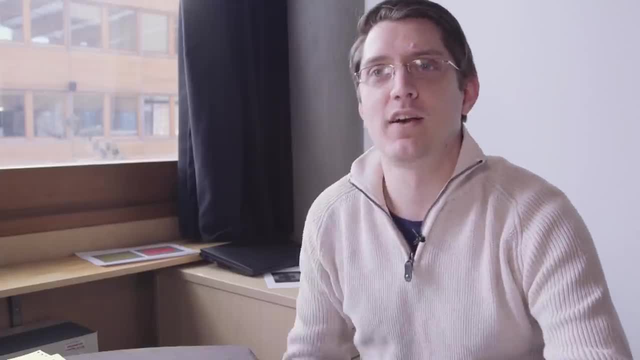 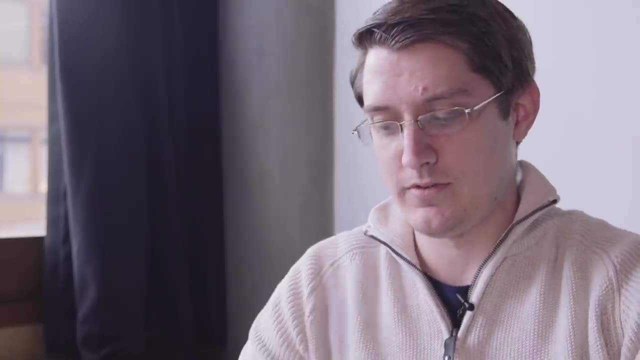 and we have our output block. And there it is. So that's the complete JPEG compression using discrete cosine transform, If we look at our input block and our output block next to each other. so there we go. we can see that there are some changes in these values. 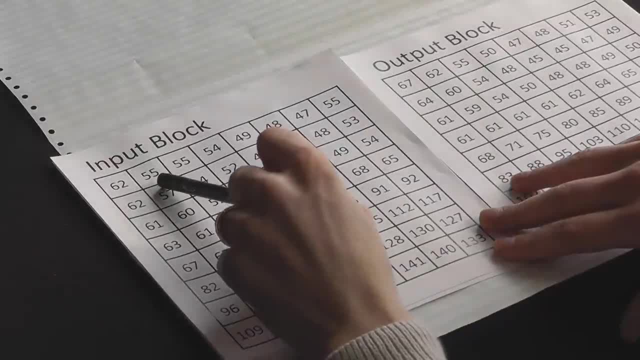 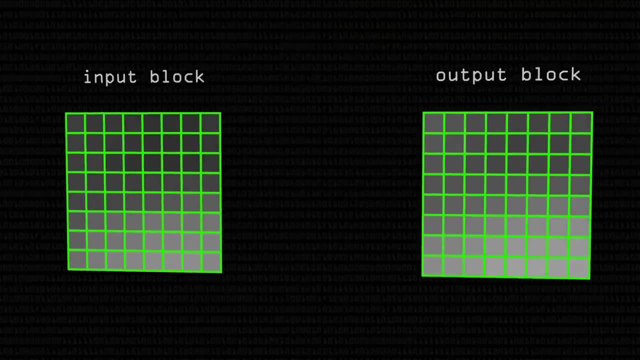 but it's actually pretty close. These have sort of changed. This has gone up a few intensity levels. This is the same. This has gone down four, But these are from nought to 255.. No one's going to see that kind of difference. 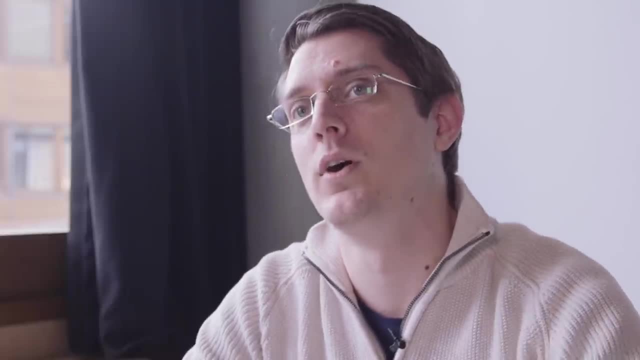 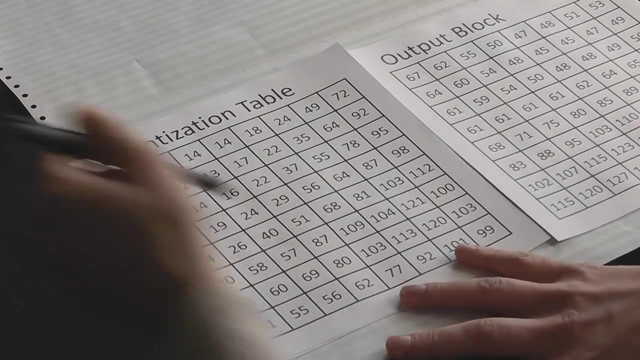 And this is at 50%. So you can do a lot less than this if you have your JPEG quality set higher and smaller values in your quantization table. So in the JPEG standard, this is the quantization table that they give you. This is actually the quantization table. 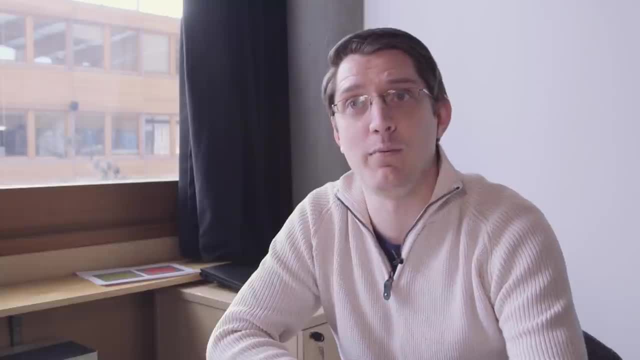 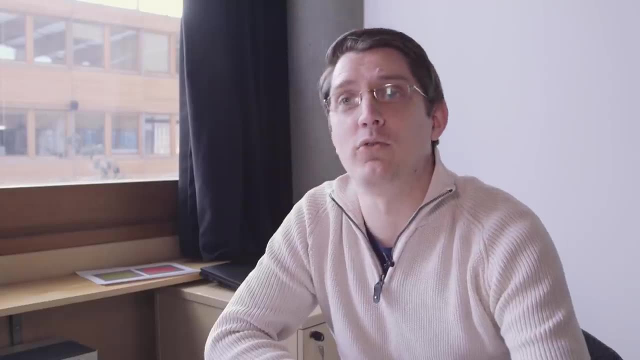 for luminosity, not for chrominance. They have a different one for chrominance, which has much higher penalties on the high frequency, Because if high frequency data is not very important, in gray it's even less important, given that we don't see color that well. 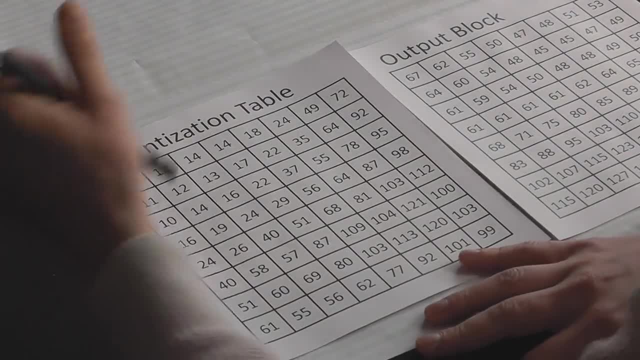 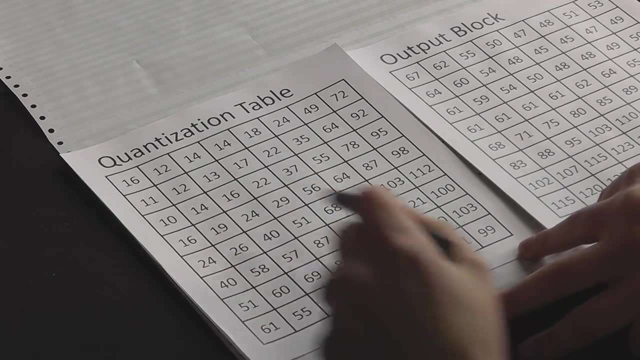 One thing that you can do to immediately increase the quality of our overall JPEG compression, that is, preserve as much image as possible, is to halve all of these values in the quantization table. If we divide all of these values by two, then essentially everything's being scaled by less. 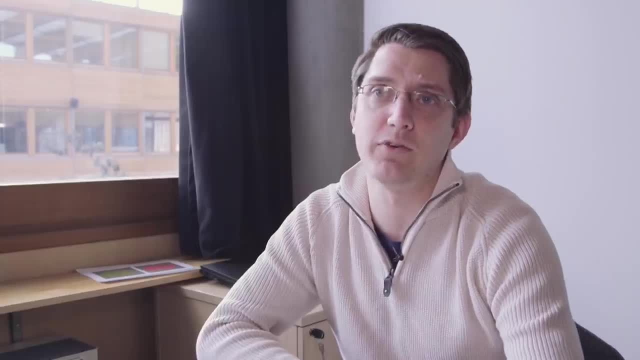 All of these high frequency quantization tables will not necessarily be rounded to zero. They might be rounded to one or two and they'll still have a little bit of an effect. On the other hand, if we increase the values in these quantization tables, 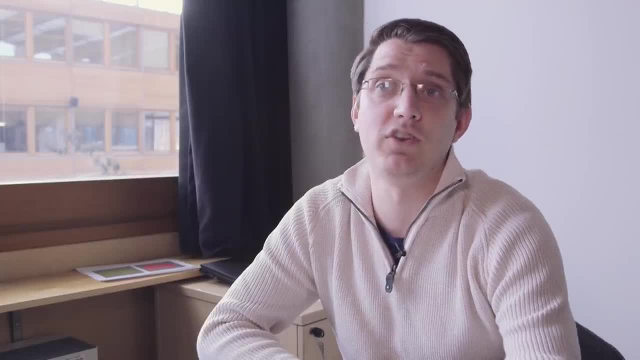 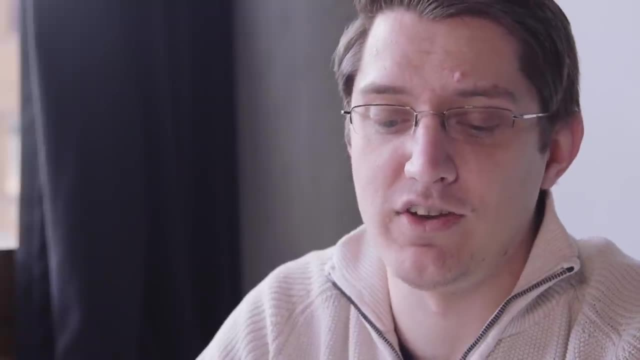 we're essentially operating a lower JPEG quality setting. This is the approach that the JPEG standard uses In other software. they may have their own quantization tables. In fact, as far as I know Photoshop, I think they have 12 quality settings. 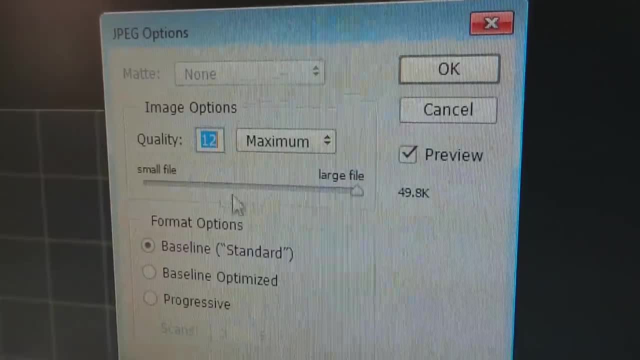 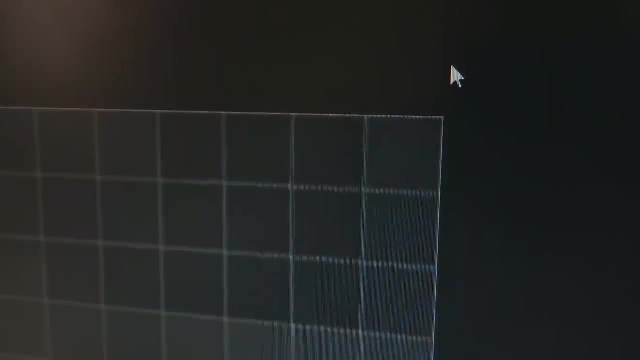 and they have different quantization tables for most of those settings and different sampling frequencies. So lots of different things that they've decided to make for a pretty good scale bar that a user can use, And all of those settings are all then stored in the header of the file. 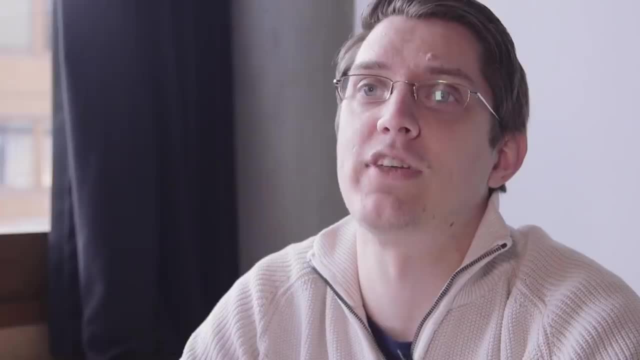 Yeah, Between each part of the image you'll get a small block that says these are the quantization tables and the Huffman coding tables that we used so that everyone can reverse that process If you don't know what the quantization table was.